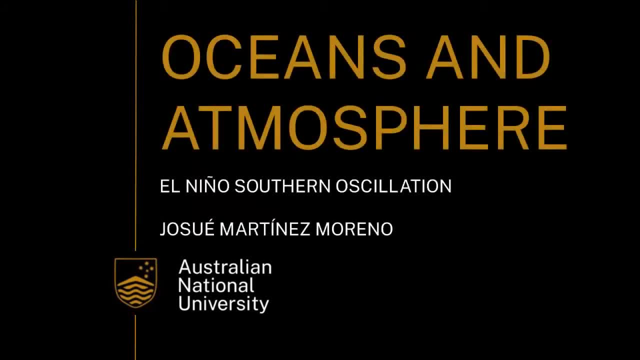 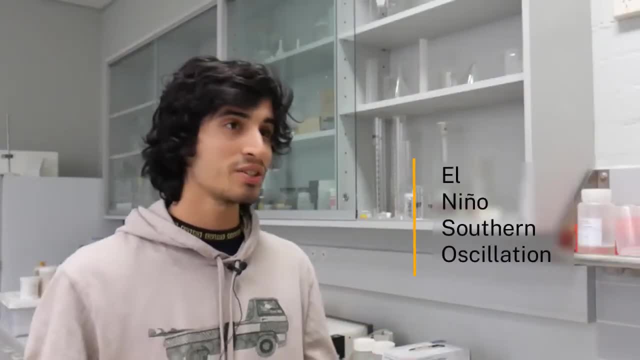 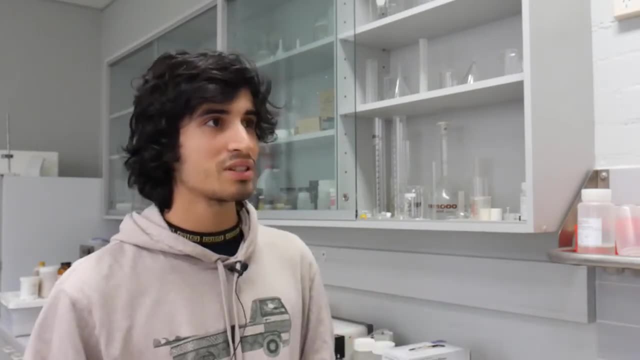 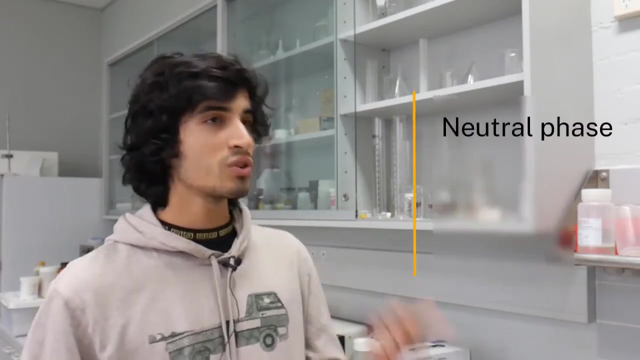 One of the best climate modes that we know of is El Niño Sudden Oscillation or ENSO. It's really important because every few years it can affect weather patterns and climate system overall. There are three phases of ENSO: Neutral phase, El Niño phase and La Niña phase. They all are interconnected and they can change how all the oceans in the earth respond to it. First of all, we started looking at what normal or neutral phase ENSO is. With everything in ENSO, it happens in the tropical Pacific. 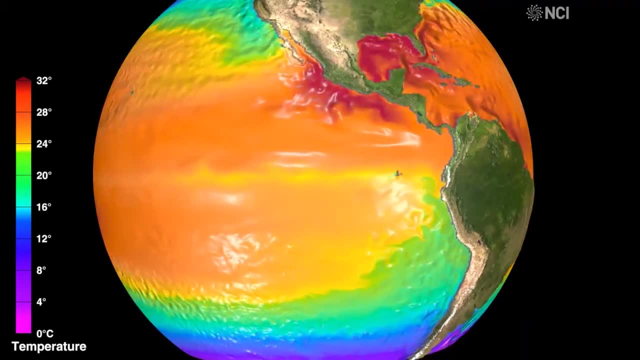 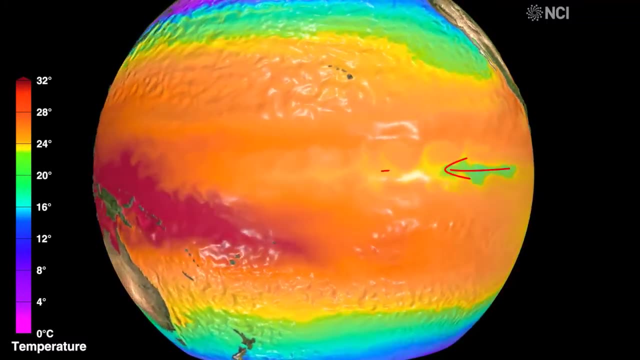 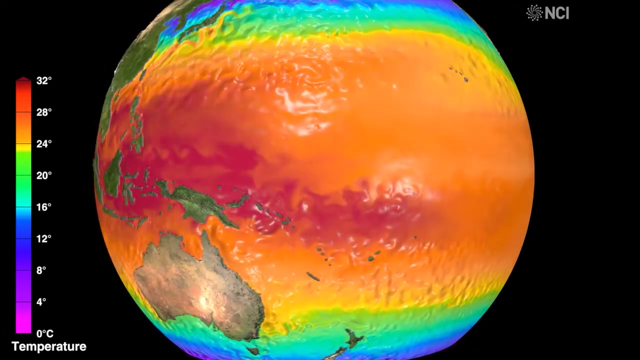 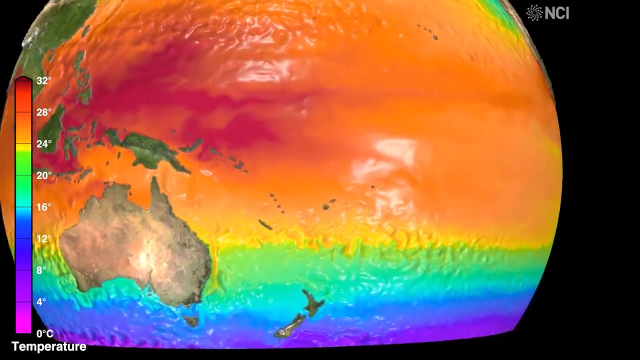 It has teleconnections to other places in the oceans, but we will focus now in the tropical Pacific. During neutral years, there's winds in the ocean. There's a tropical Pacific that flows from America to Australasia. These winds have the peculiarity that they can move the surface of the ocean, which is warm, to the west. 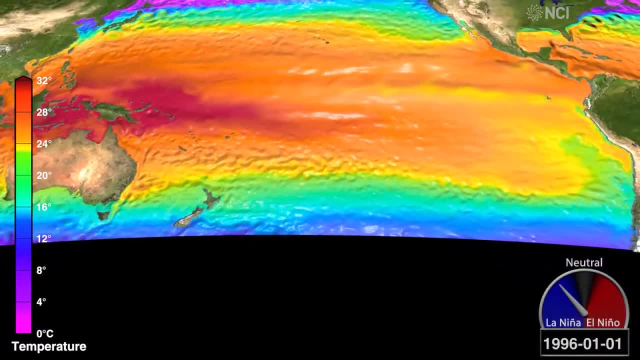 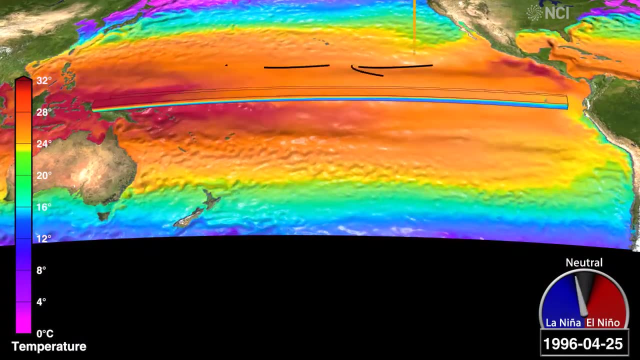 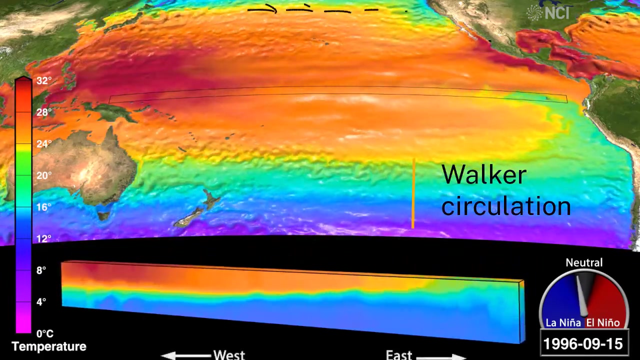 That creates this warm pool of water, which, in consequence, generates moisture and hot air that rises up. It creates this circulation that is called the Walker circulation. This is really important because it also feeds back into keeping and maintaining this neutral phase as the winds flow from the east to the west. 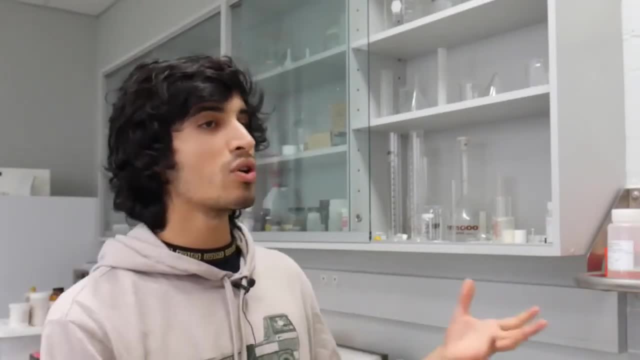 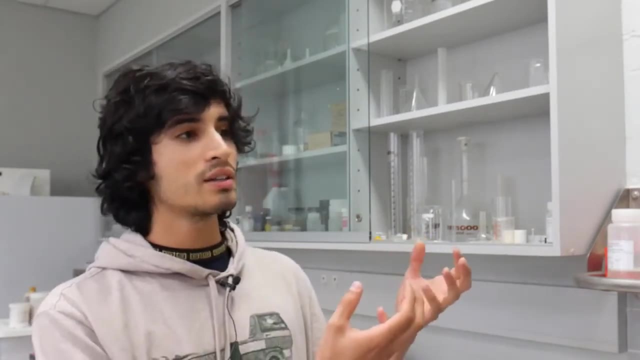 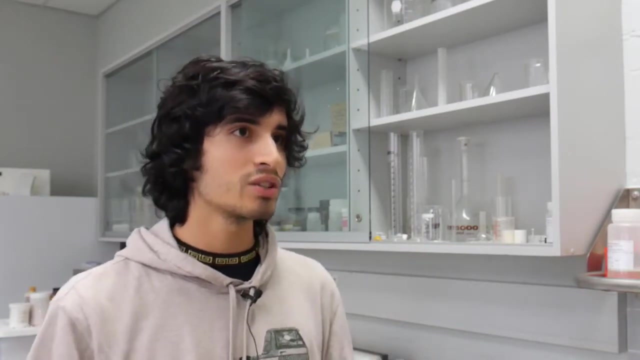 These great winds have the peculiarity that they will pile up this water on the western side of the tropical Pacific Ocean. As a consequence of that, there will be water rising from the deeper layers of the ocean in the east side of the tropical Pacific. 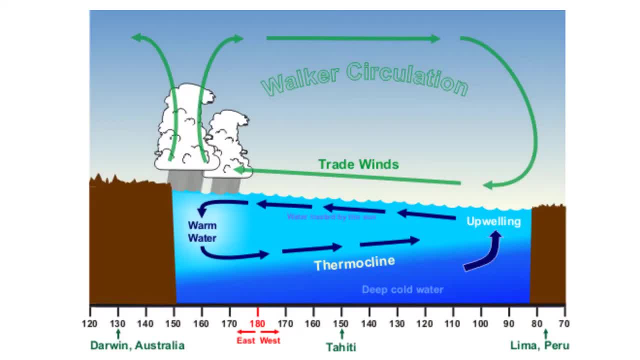 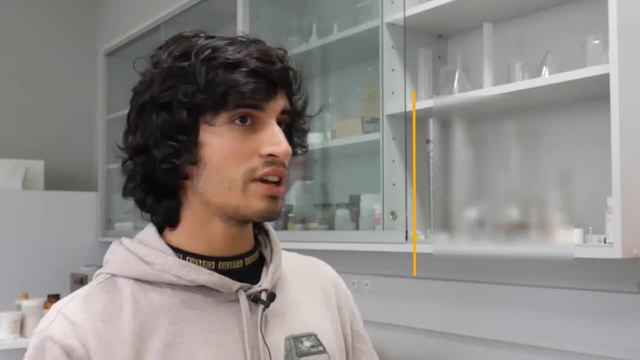 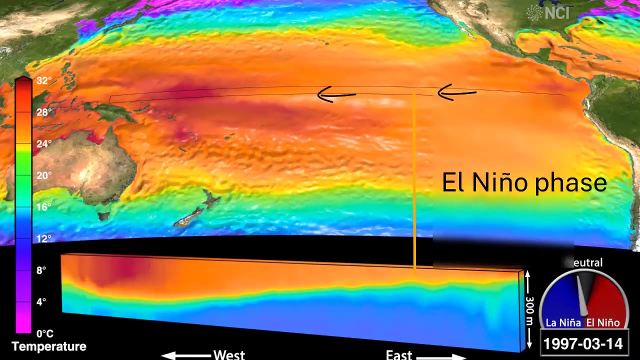 That process is known as a boiling. Now that we understand the neutral phase, we'll move on into what El Niño phase represents. All El Niño phases start with a weakening of the great winds. As soon as the great winds weaken, which means that the east to west flow of the winds decrease, 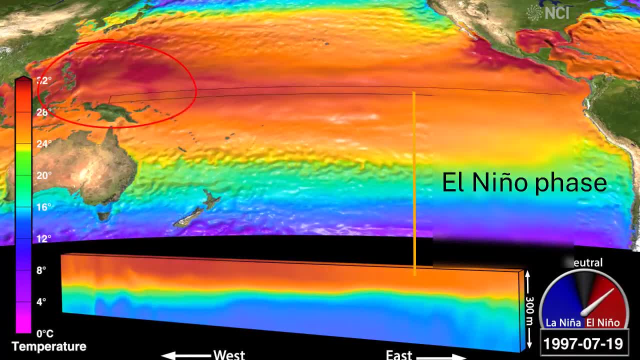 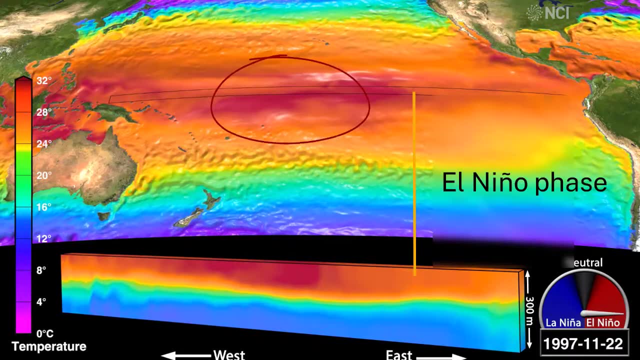 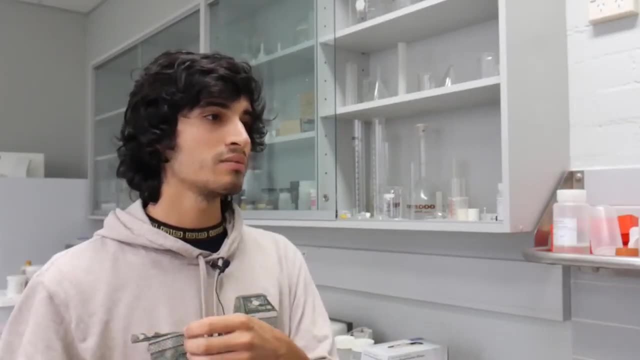 this warm pool of water that was already piled up in the western side of the tropical Pacific Ocean can move now into the central ocean- This is the central Pacific- or to the east Pacific. That also occurs in conjunction with the surface water in those other regions staying warm. It's now not being pushed to the west. As soon as that happens, then this location where the water can affect the atmosphere changes. If it moves to the central Pacific, then hot water and humid water will rise up there. Then that will mostly mean that the precipitation in the tropical Pacific will occur within the ocean.